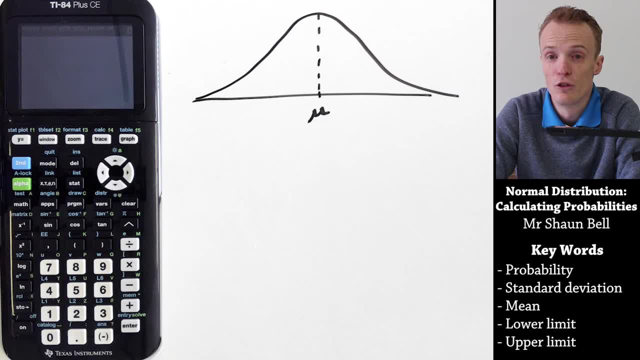 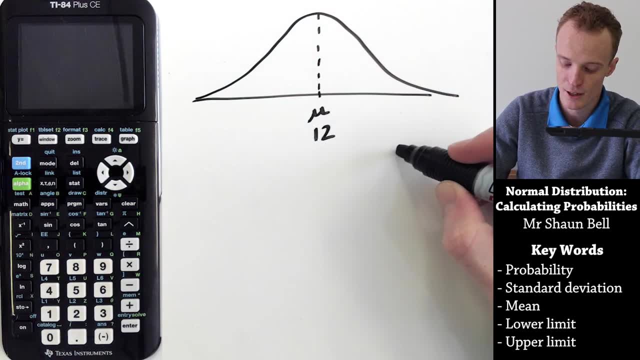 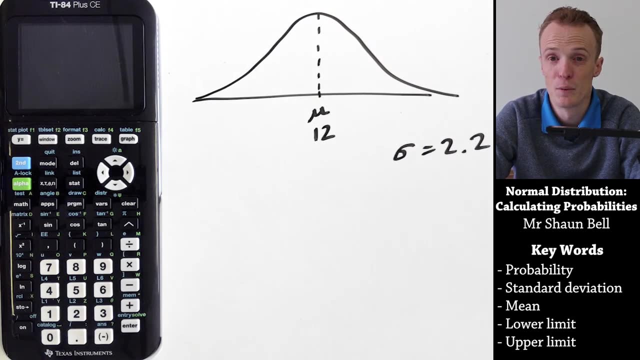 cookies and this graph represents the number of choc chips on each cookie and the mean here will say is 12, and it has a standard deviation which is equal to 2.2.. And let's pretend that we're aiming for each cookie to have between 8 and 14 choc chips. What we're essentially trying to do, 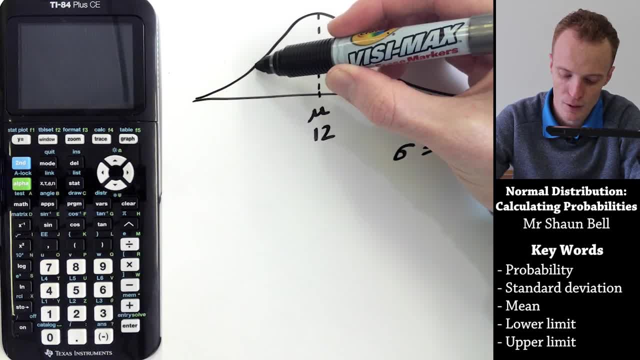 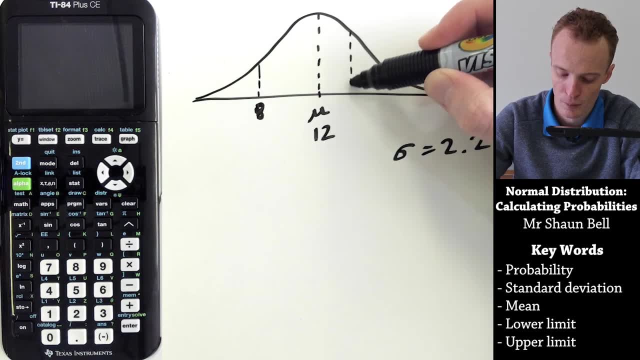 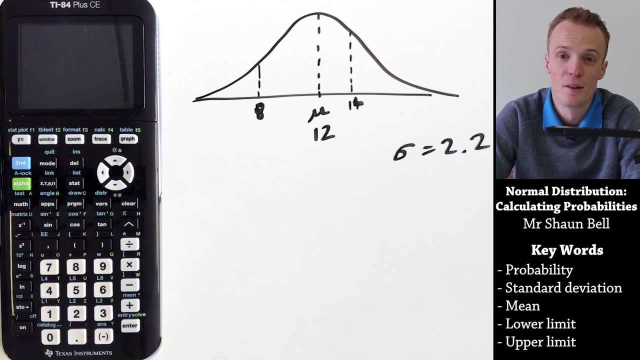 is, we're trying to work out how many of the cookies are going to be between this 8 here and the 14 which would approximately be in here. Well, to be able to do that, we would first need to be able to calculate the probability of each. 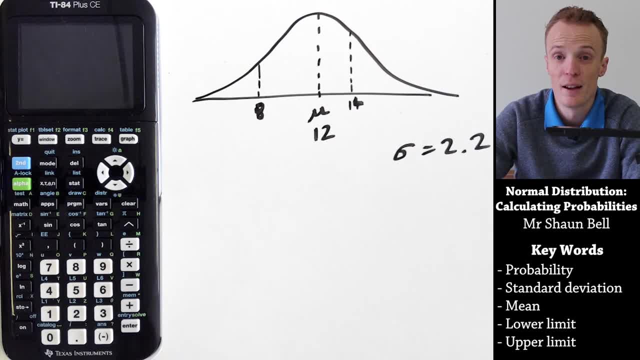 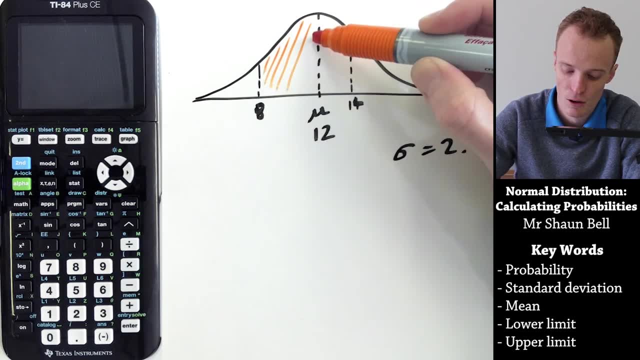 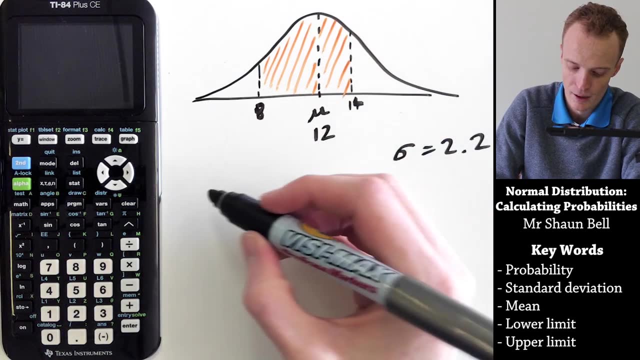 cookie falling between these ranges and when we're calculating probability using a normal distribution, we're actually calculating the area that is inside of what we've just stated. So if we were to calculate the probability that our cookie, which I'm just going to use, X to, 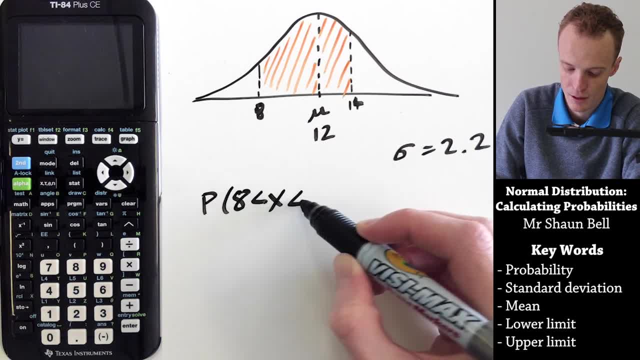 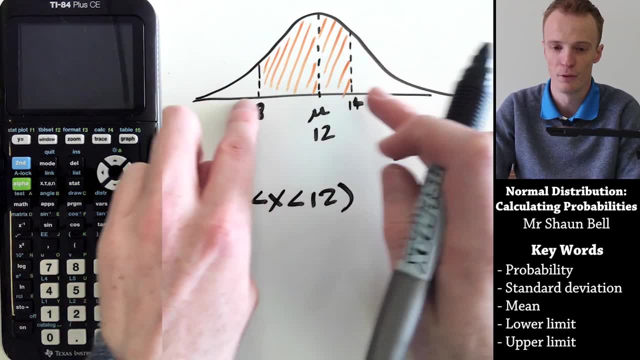 represent is between 9 and 14 choc chips. So we would calculate the probability of an actual between 8 and 12,. we would find the chance of any individual cookie falling between this region of our graph. All right, so let's now enter this into our calculator To do that. just make sure. 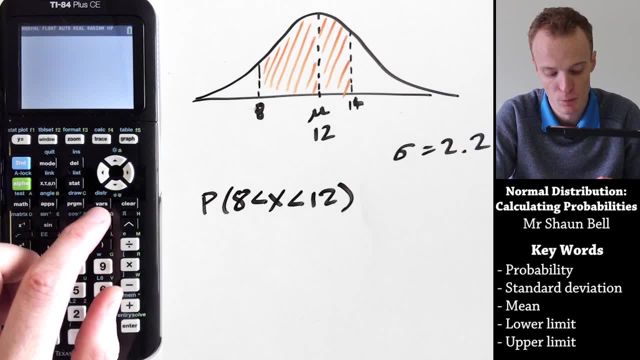 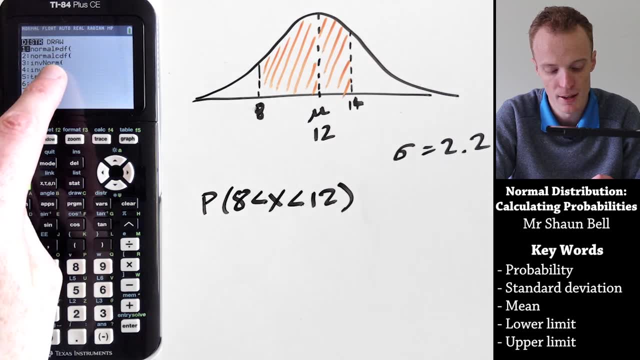 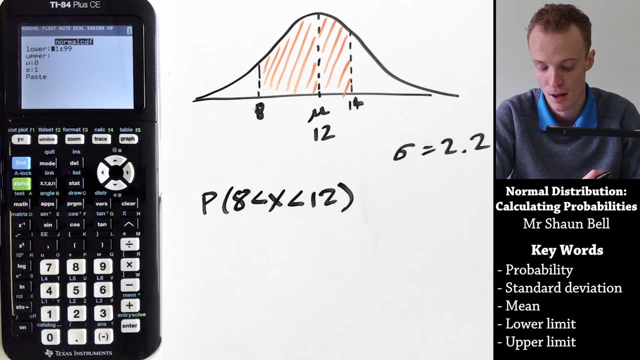 your calculator is on And we want to go to the distribution section which is above the VAS button. So we go to second distribution And the one that we want is normal CDF, which is option 2.. So you can scroll down and press enter And it'll ask us for the lower and upper bound, The 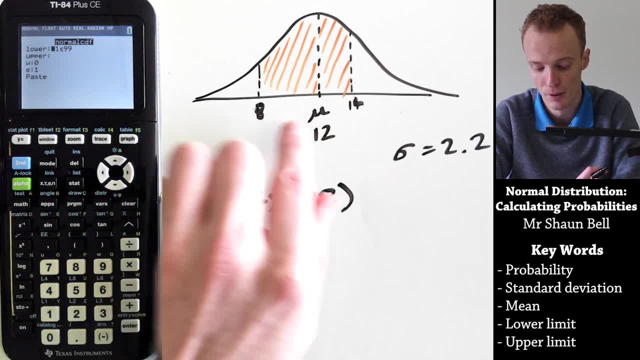 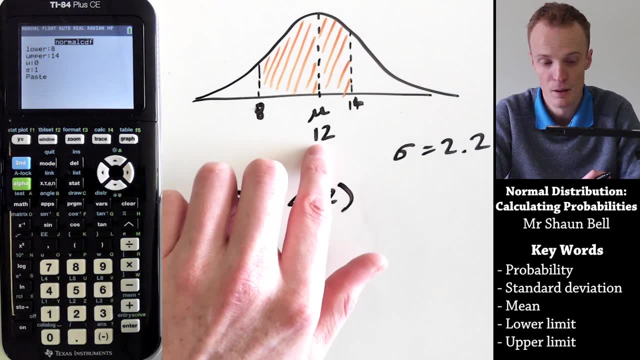 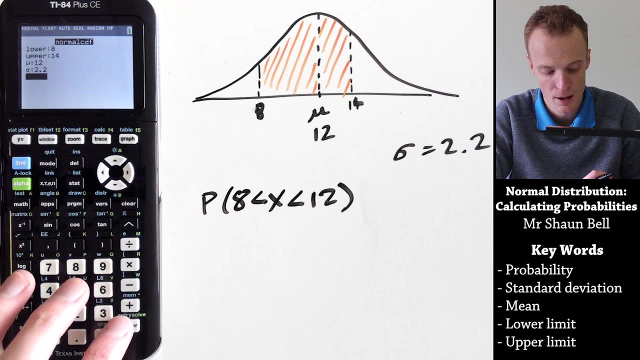 lower and upper bound is represented in here, this one being our lower, this one being our upper. So our lower is 8,, our upper is 14.. Then it'll ask for our mean, which here is 12, and our standard deviation, which here is 2.2.. And we hit the paste and it'll put it into our 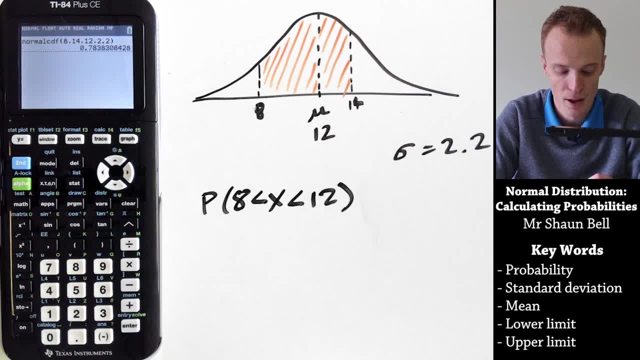 run screen. Now we hit the enter again and it'll give us the standard deviation, which here is 2.2. And we hit the paste and it'll put it into our run screen. Now we hit the paste and it'll give us the probability of it falling between these. 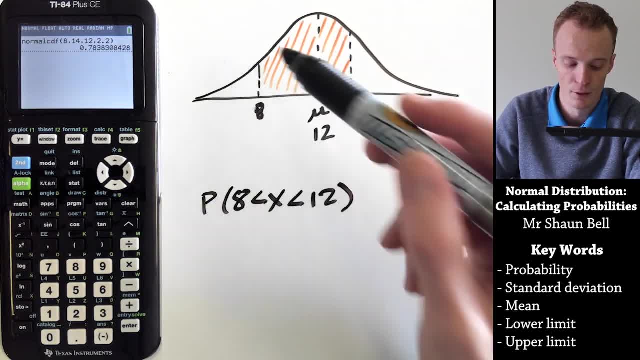 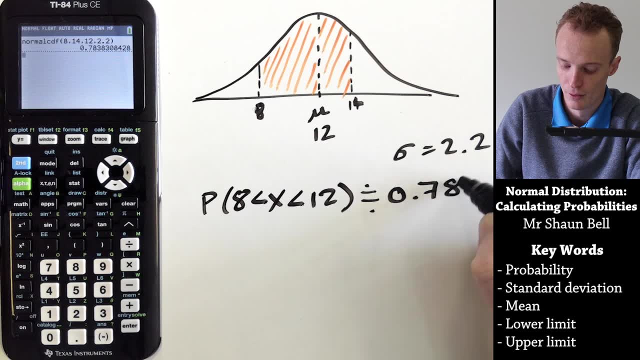 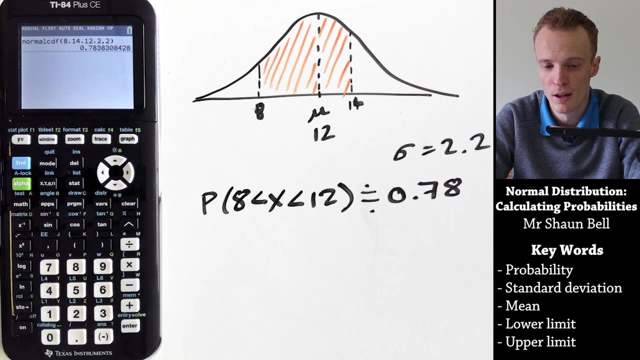 two values, which is also the area underneath this graph. So our probability is approximately equal to 0.78.. What that means is there's approximately a 78% chance of each cookie having between 8 and 14 choc chips on there, But let's say that I wanted to make sure that I had. 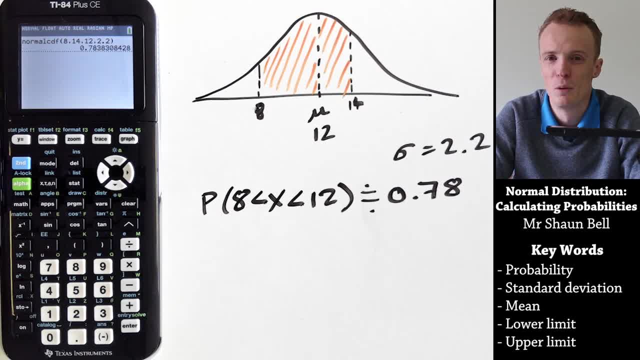 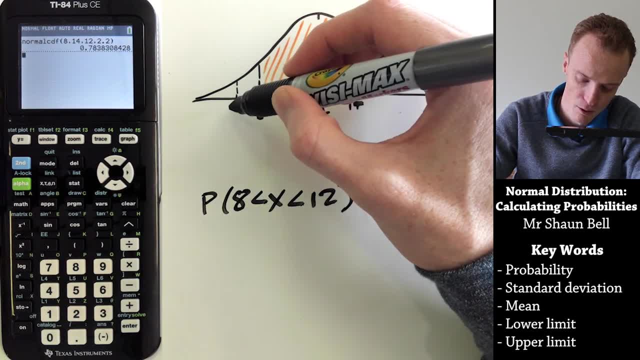 at least six choc chip cookies on there, And I wanted to make sure that I had at least six choc cookies on there. So what I want to know is: what is the chance of getting less than six? So six would probably be approximately here on my graph. I want to know what the area is inside of this. 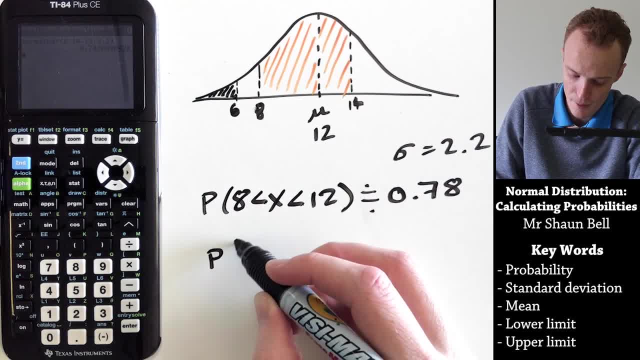 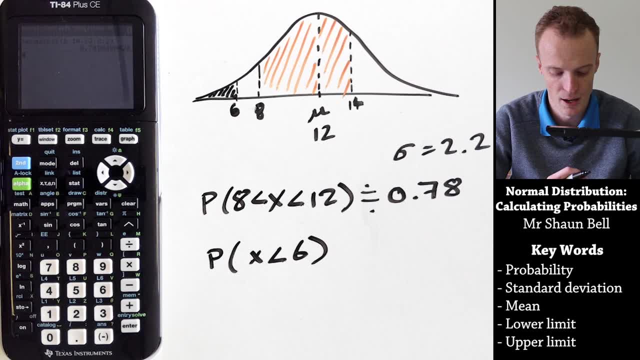 in black. So the probability that my x value is less than six. Now, to enter this into your calculator, you go back into the distribution CDF function. so normal CDF, as we did before. But we now need to change the lower function And we need to. 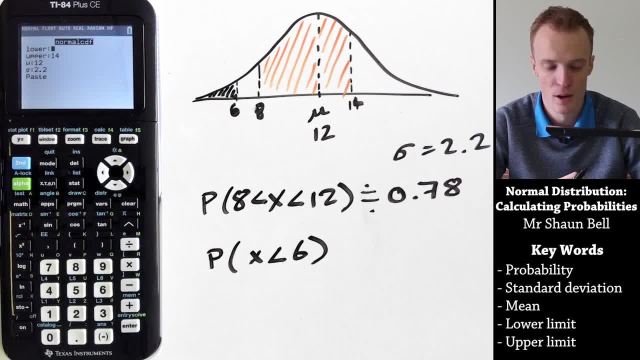 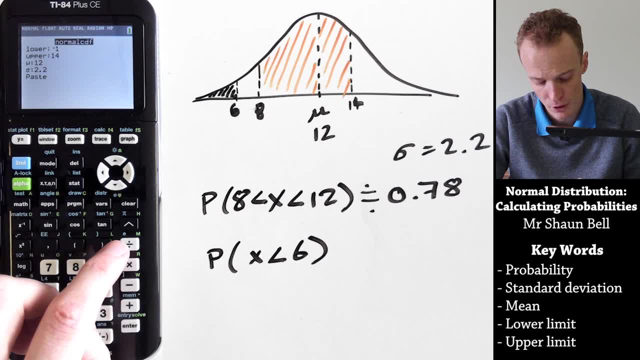 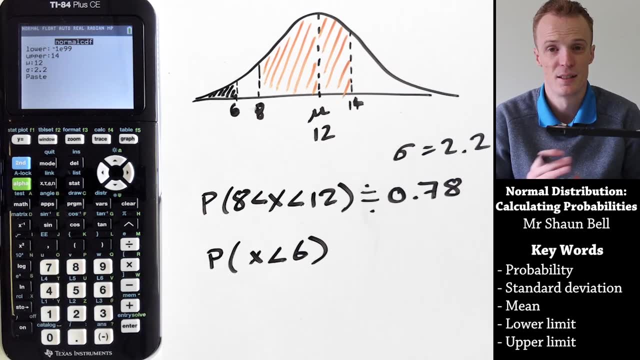 change the lower function to a really, really small number. Now, to do this, we usually go negative 1 to the e, which is that value above the divide sign. So you go second e to the 99. And what that indicates is it's infinitely negative inside of our calculator. Our upper bound is the 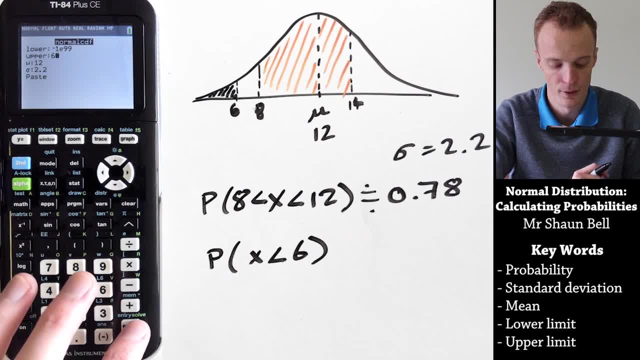 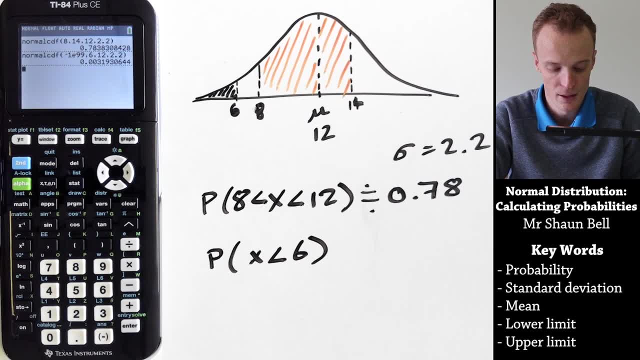 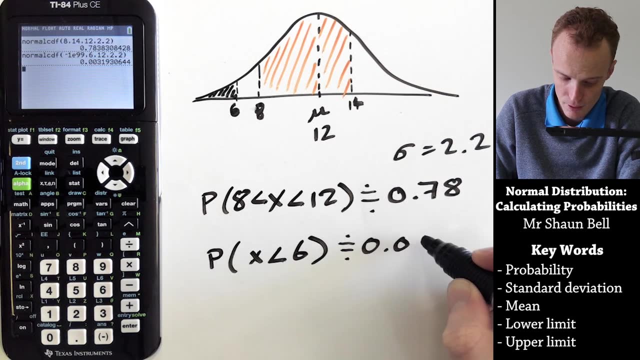 six. We don't want it to go any higher than the six, So we put our six in. Our mean and our standard deviation are the same, So we paste that in and then hit the enter And it will tell us that the probability is approximately equal to 0.0032.. So the key thing is if we're dealing with a 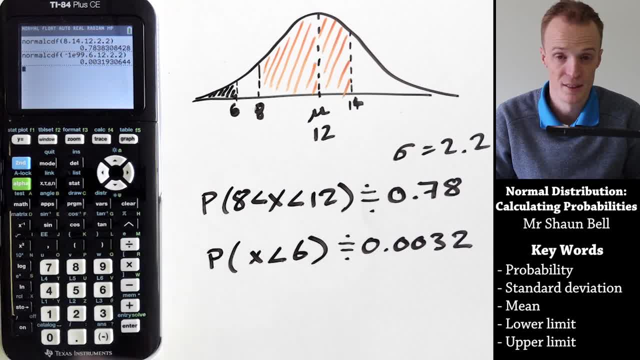 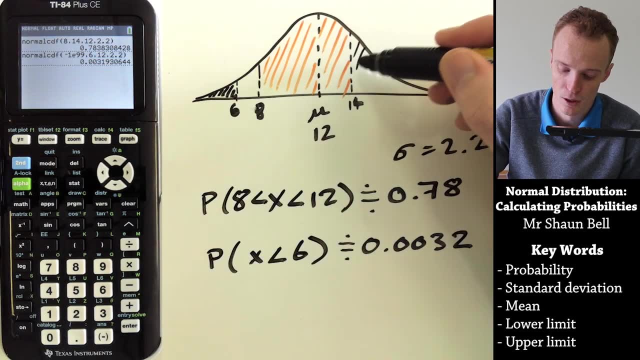 probability that's got no lower limit, and the same thing for an upper limit. we need to put into our calculator a value that's really really small or a value that's really really large, For example if I want to know the chance of getting one that's higher than 14 here. so this area in here.